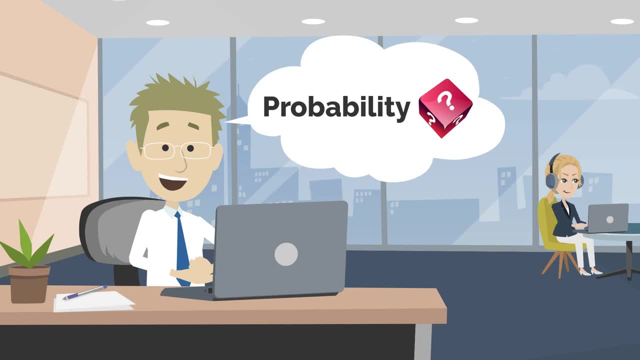 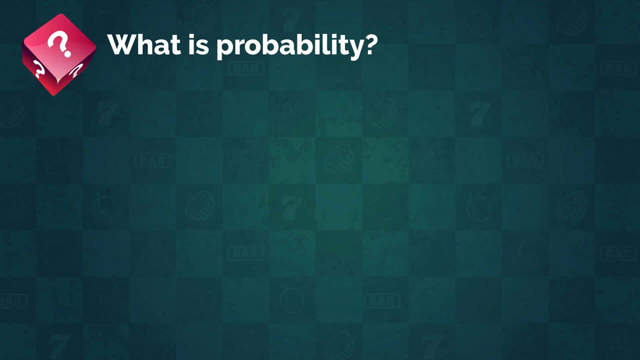 they can predict how likely each outcome is and make the right call for their firm. Some of you might be wondering: what is this probability we're talking about? Essentially, probability is the chance of something happening. A more academic definition for this would be the likelihood of an event occurring. 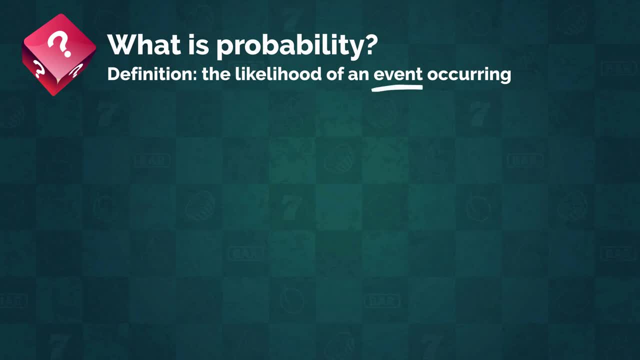 The word event has a specific meaning when talking about probabilities. Simply put, an event is a specific outcome or a combination of several outcomes. These outcomes can be pretty much anything: Getting heads when flipping a coin, rolling a four on a six-sided die or running a mile in under six minutes. 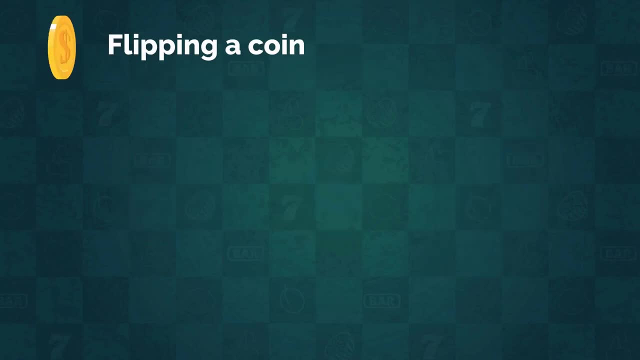 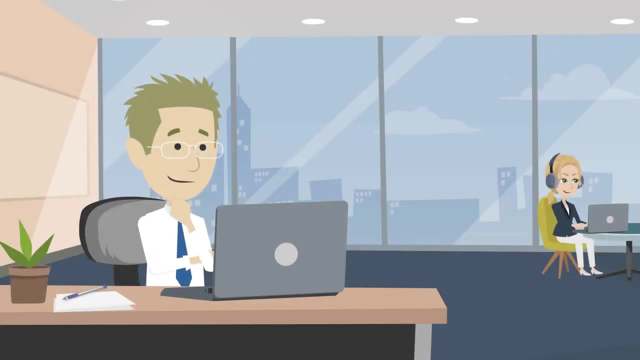 Take flipping a coin, for example. There isn't only one single probability involved. There are two possible outcomes: Getting heads or getting tails. That means we have two possible events and we need to assign probabilities to each one. When dealing with uncertain events, we are seldom satisfied by simply knowing whether 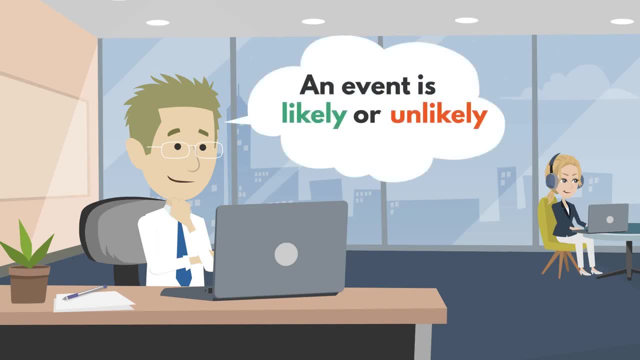 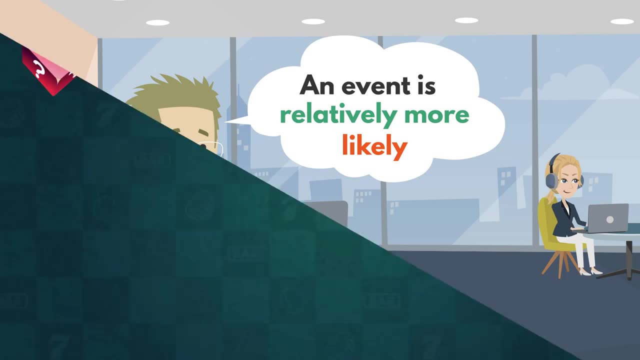 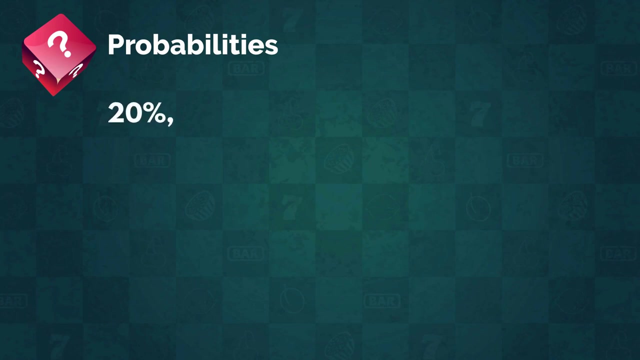 an event is likely or unlikely. Ideally, we want to be able to measure and compare probabilities in order to know which event is relatively more likely. To do so, we express probabilities numerically, Even though we can express probabilities as percentages or fractions conventionally. we 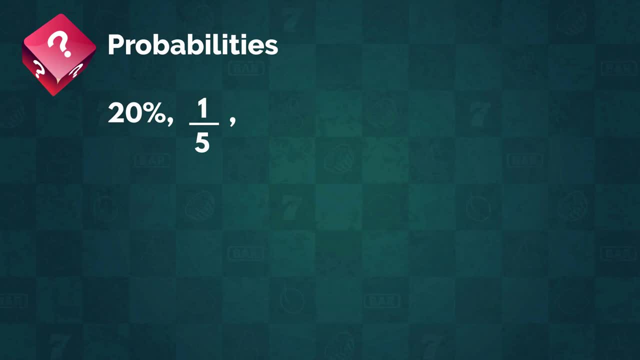 write them out using real numbers between 0 and 1.. So, instead of using 20% or one fifth, we prefer .2.. Alright, now let us briefly talk about interpreting these probability values. Having a probability of 1 expresses absolute certainty of the event occurring And a probability of zero. 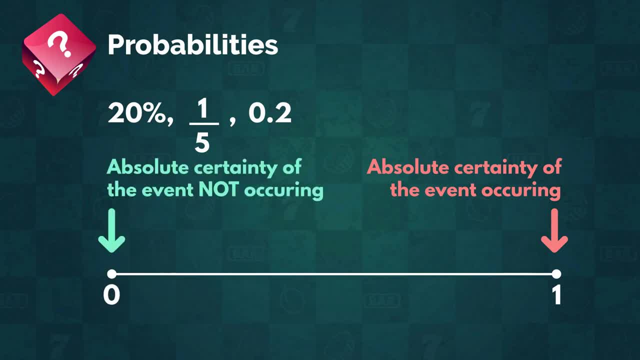 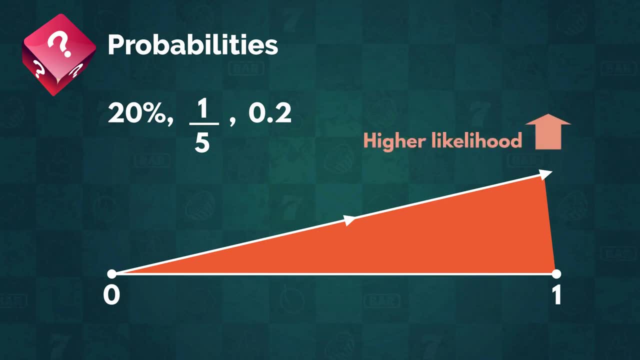 expresses absolute certainty of the event not occurring. You probably figured this out, but higher probability values indicate a higher likelihood. Okay, as you can imagine, most events we are interested in would have a probability other than zero and one, So values like 0.2,, 0.5, and 0.66. 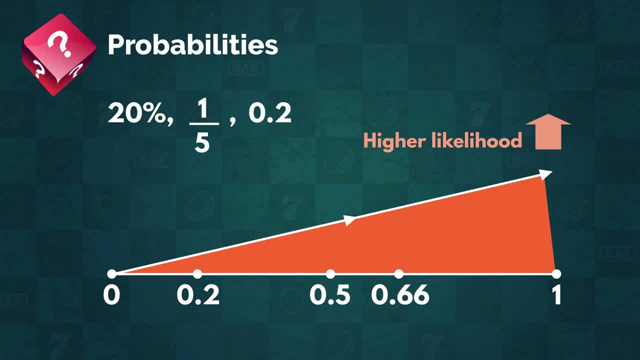 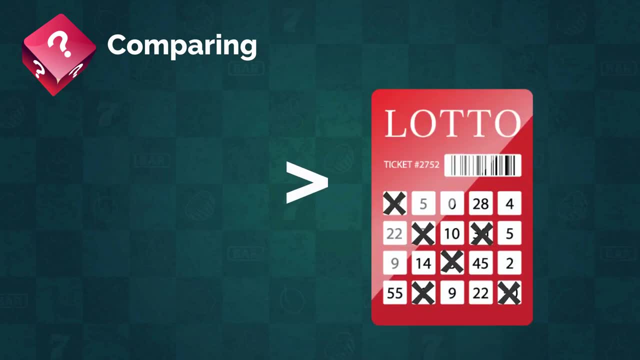 are what we generally expect to see. Even without knowing any of this, you can tell some events are more likely than others. For instance, your chance of winning the lottery isn't as great as winning a coin toss. That's why you can think of probability. 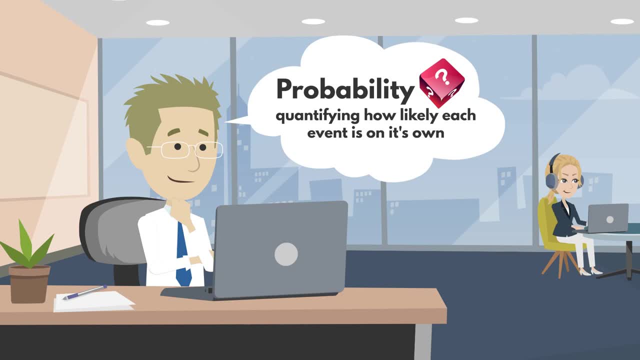 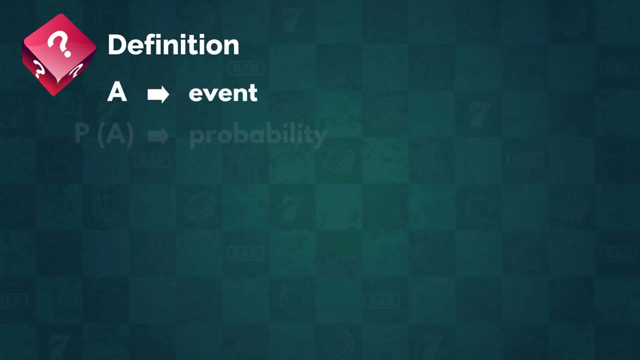 as a field. that is about quantifying exactly how likely each of those events are on their own. So how about we start right away? Let's get into it. Generally, the probability of an event A occurring, denoted P of A is equal to the number. 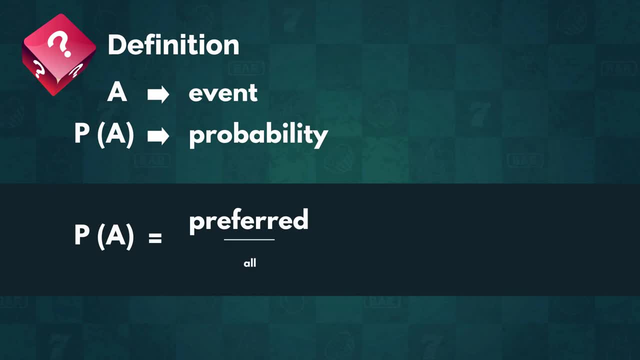 of preferred outcomes over the total number of possible outcomes. By preferred we mean outcomes that we want to see happen. A different term people use for such outcomes is favorable. Similarly, sample space is a term used to depict all possible outcomes Going forward. we shall use the respective terms. 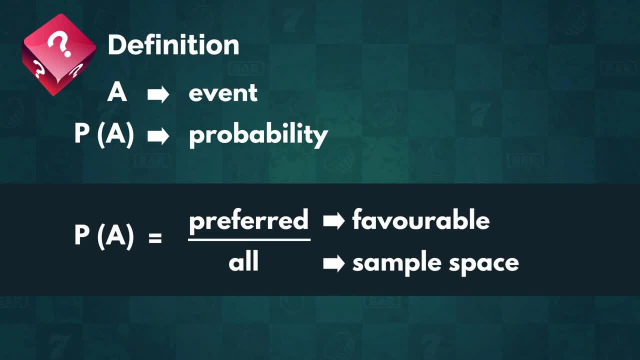 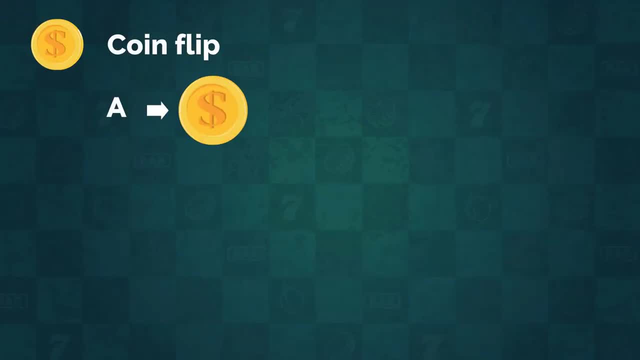 interchangeably. We will go through several examples to ensure you understand the notion. well, Say, event A is flipping a coin and getting heads. In this case, heads is our only preferred outcome, Assuming the coin doesn't just somehow stay in the air indefinitely. 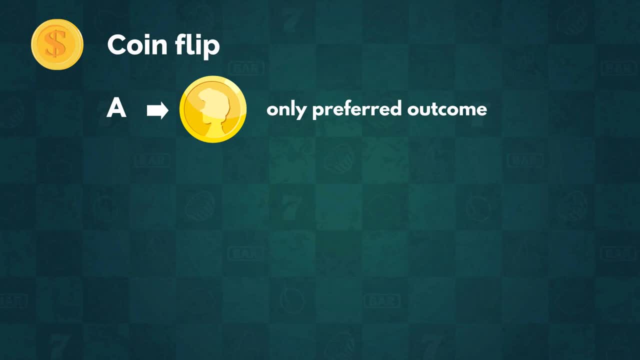 there are only two possible outcomes: heads or tails. This means that our probability would be a half. so we write the following: P of getting heads equals one half, which equals one half, Which equals 0.5.. All right. Now imagine we have a standard six-sided die. 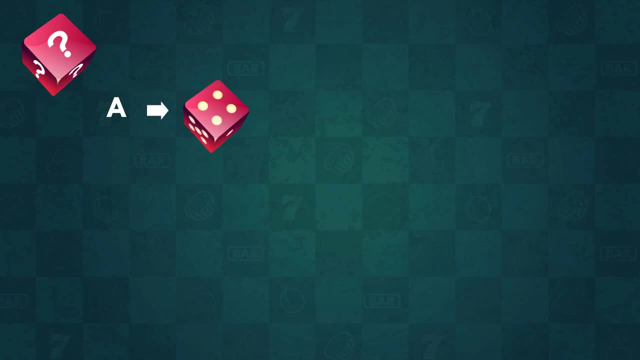 and we want to roll a four. Once again, we have a single preferred outcome, But this time we have a greater number of total possible outcomes: six. Therefore, the probability of this event would look as follows: P of rolling four equals one sixth. 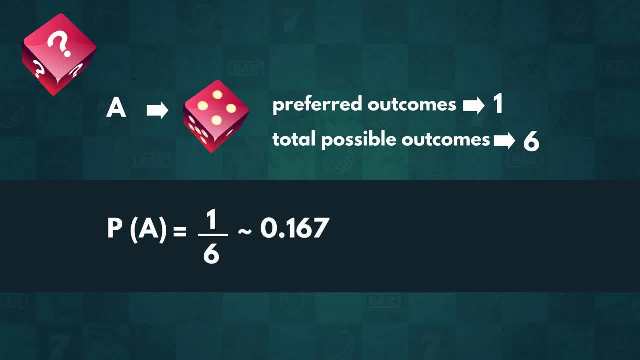 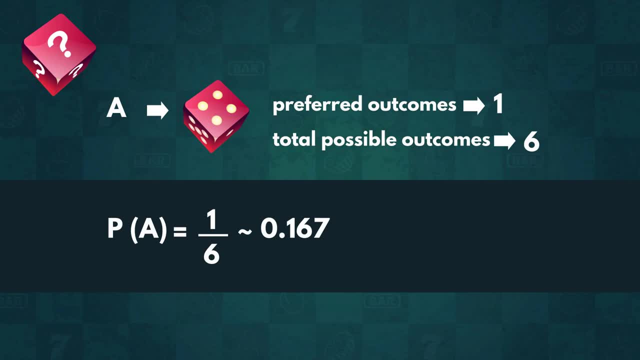 P of rolling four equals one sixth, or approximately 0.167.. P of rolling four equals one sixth, or approximately 0.167.. Great Events can be simple or a bit more complex. For example, what if we wanted to roll a number divisible by three? 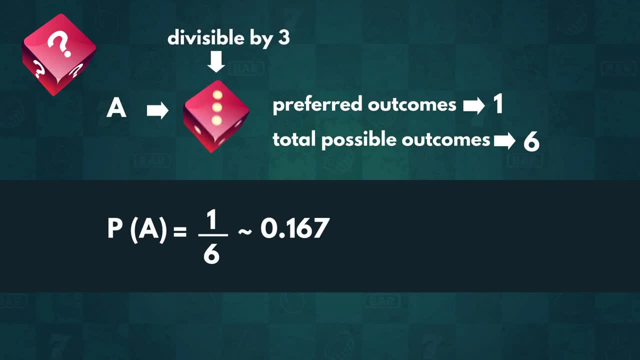 That means we need to get either a three or a six, so the number of preferred outcomes becomes two. However, the total number of possible outcomes stays the same, since the die still has six sides. Therefore, we conclude that the probability of rolling a number divisible by three equals two over six. 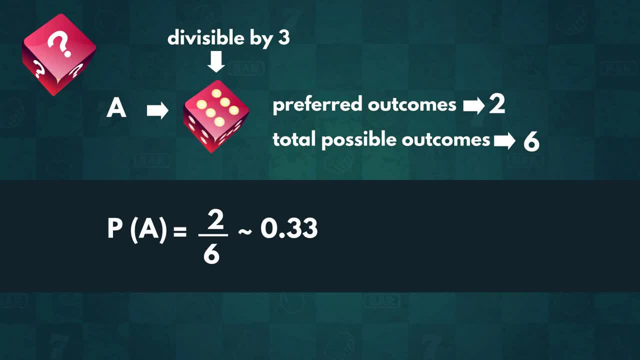 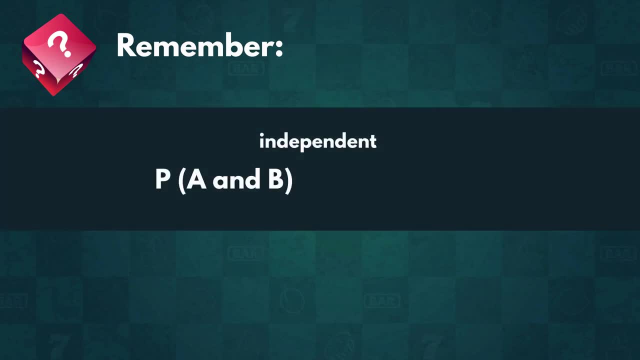 which is approximately 0.33.. So far, so good. Note that the probability of two independent events occurring at the same time is equal to the product of all the probabilities of the individual events, For instance, the likelihood of getting the ace of spades. 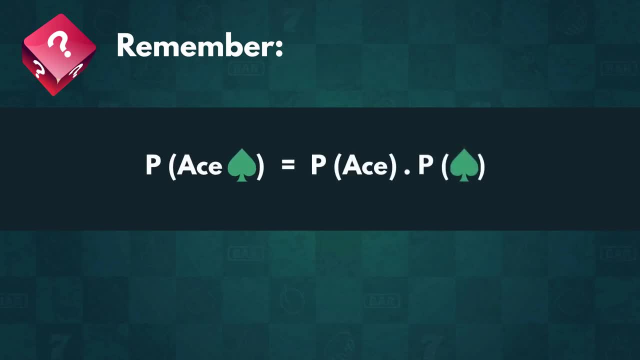 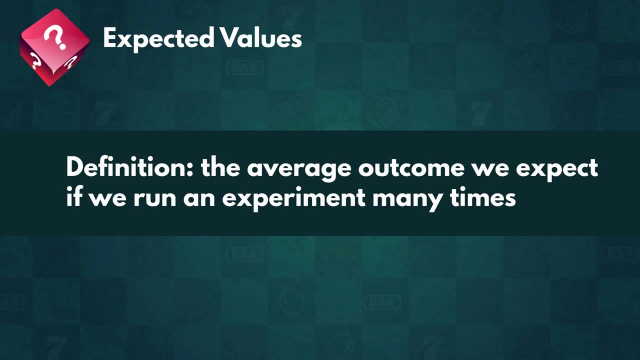 equals the probability of getting an ace times the probability of getting a spade. Expected values represent what we expect the outcome to be if we run an experiment many times. To fully grasp the concept, we must first explain what an experiment is Okay. 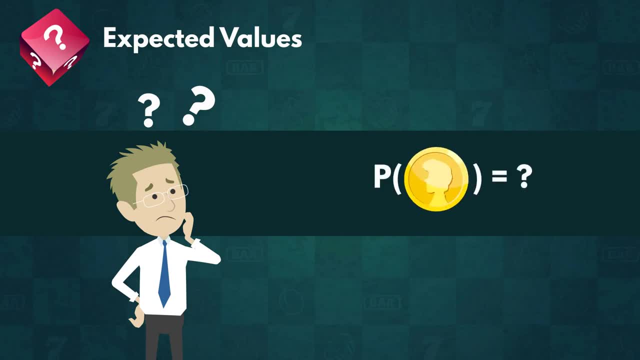 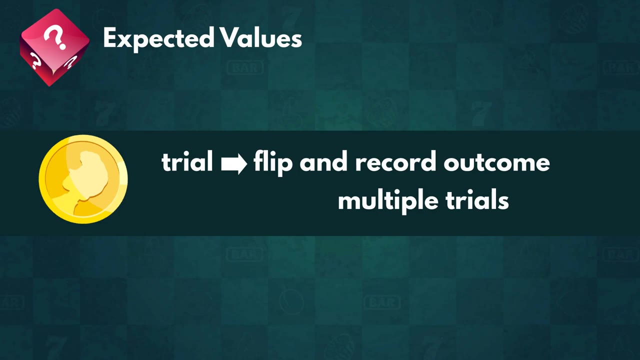 Imagine we don't know the probability of getting heads when flipping a coin. We are going to try to estimate it ourselves. So we toss a coin several times. After doing one flip and recording the outcome, we complete a trial By completing multiple trials. 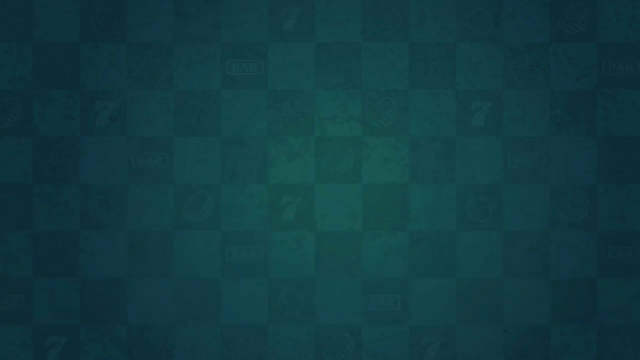 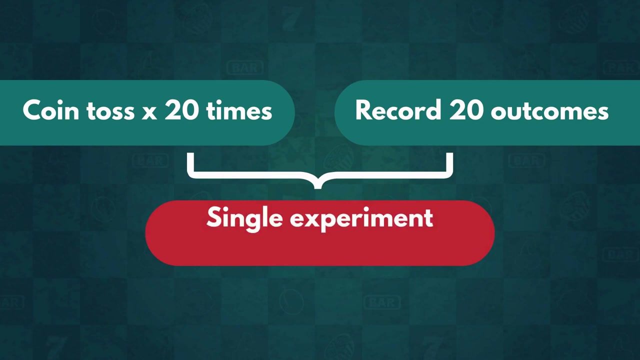 we are conducting an experiment. For example, if we toss a coin twenty times and record the twenty outcomes, that entire process is a single experiment with twenty trials. Alright, The probabilities we get after conducting experiments are called experimental probabilities, whereas the ones we introduced earlier. 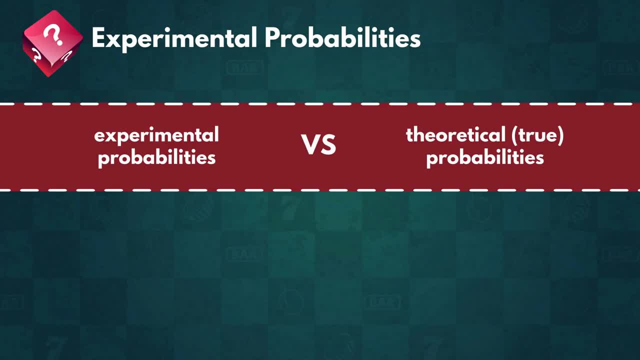 were theoretical or true probabilities. Generally, when we are uncertain what the true probabilities are or how to compute them, we like conducting experiments. The experimental probabilities we get are not always equal to the theoretical ones, but are a good approximation. For instance, 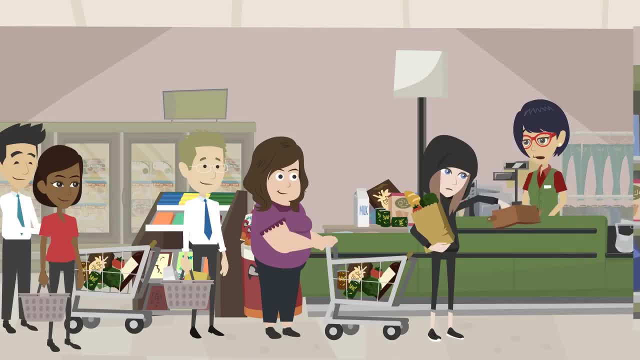 eight out of ten times I go to my local shop I have to wait in line. Based on my experience, eighty percent of the time there will be a queue and twenty percent of the time there won't be one. I can try to calculate the true probability. 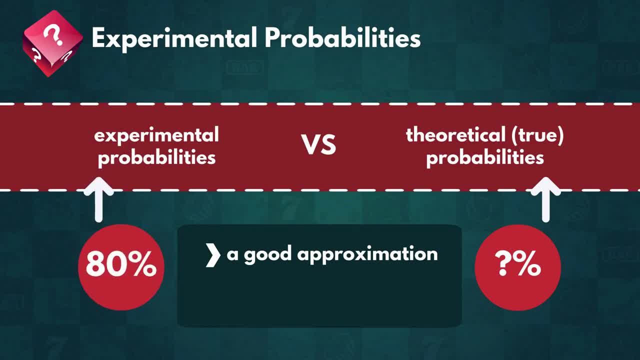 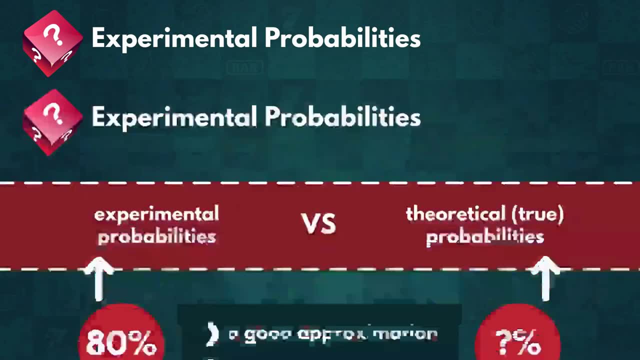 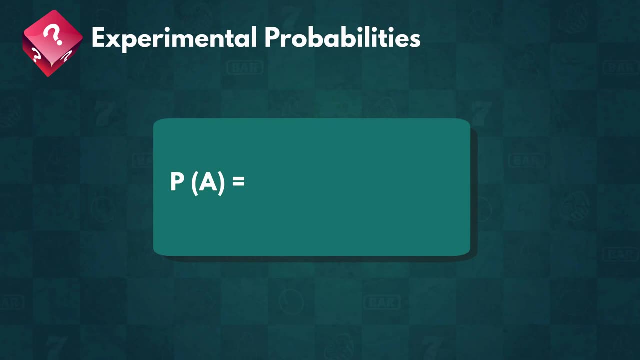 but it would include far too many factors. The experimental probability, on the other hand, is easy to compute and very useful. Okay, The formula we use to calculate experimental probabilities is similar to the formula applied for the theoretical ones earlier in the course. 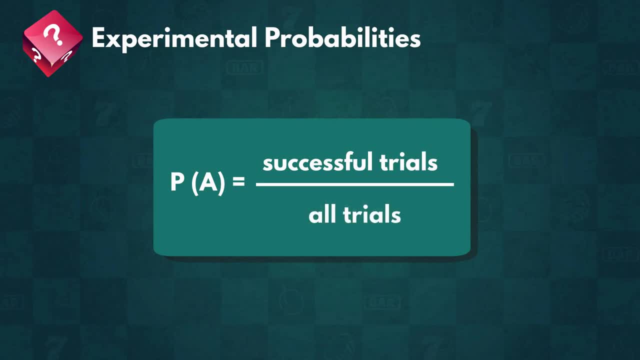 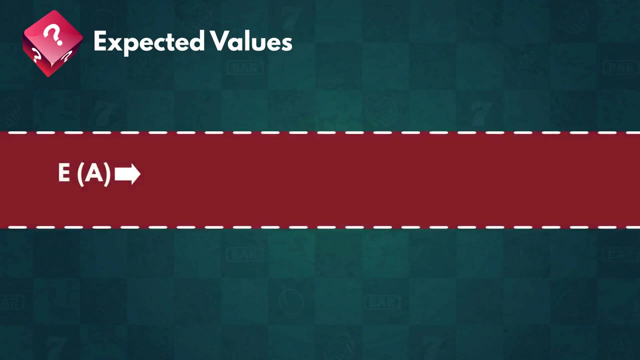 It is simply the number of successful trials divided by the total number of trials. Now that we know what an experiment is, we are ready to dive into expected values. The expected value of an event- A, denoted E of A- is the outcome we expect to occur. 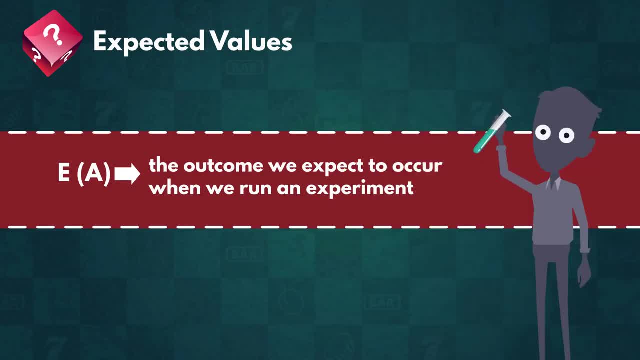 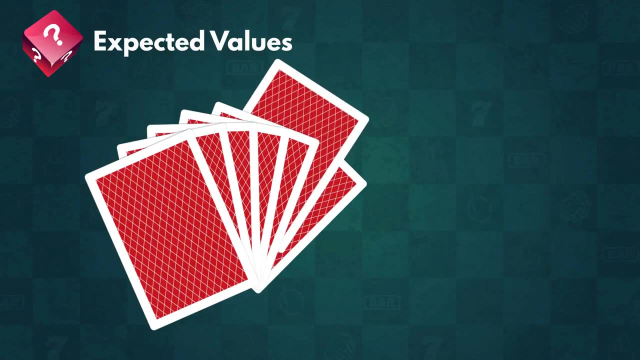 when we run an experiment. To clarify any confusion around the definition, let us examine the following example. We want to know how many times we will get a spade if we draw a card twenty times. We always record the value of a card and then return it to the deck. 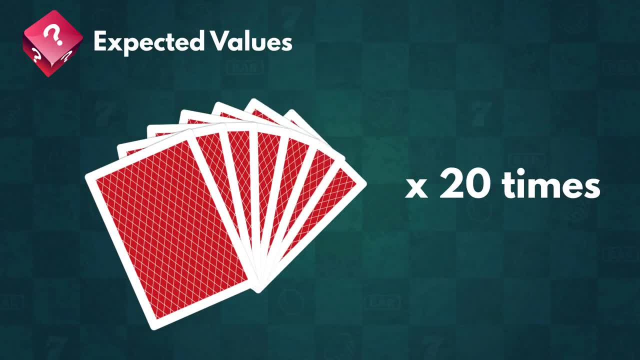 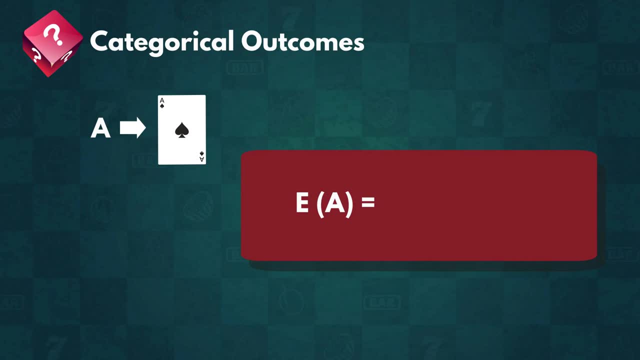 before shuffling For an event with categorical outcomes, like suits, we calculate the expected value by multiplying the theoretical probability of the event P of A by the number of trials we carried out. N. We've already seen how to compute the true probability of drawing a card. 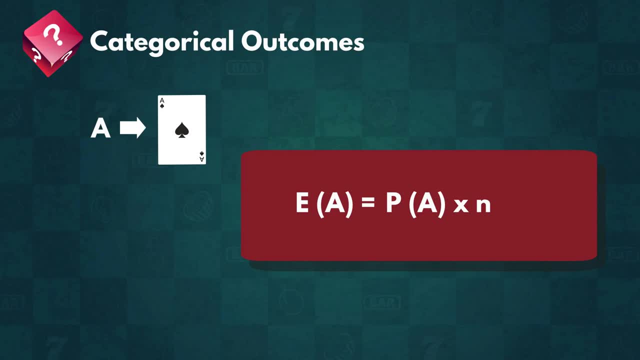 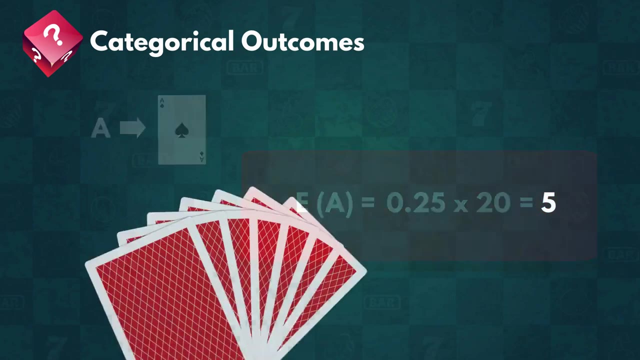 from a specific suit. It is equal to one-fourth or 0.25.. If we repeat this action twenty times, the expected value would equal 0.25 times 20, which equals five. An expected value of five means we expect to get a spade five times. 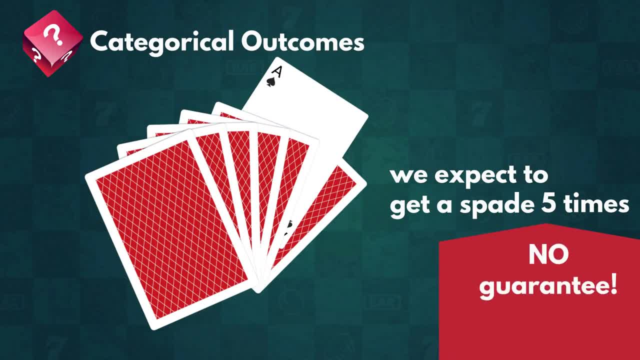 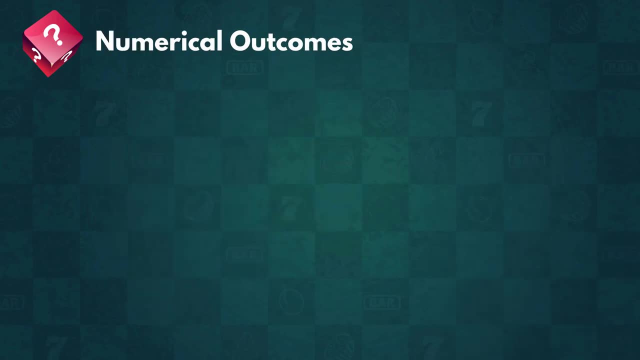 if we run the experiment, However, nothing guarantees us getting a spade exactly five times. Realistically, we could get a spade four times, six times or even twenty times. Now for numerical outcomes, we use a slightly different formula. 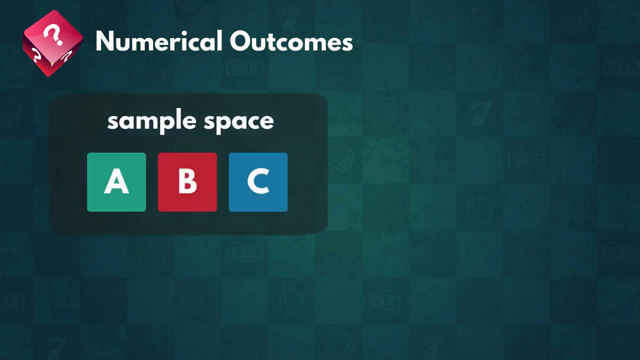 We take the value for every element in the sample space and multiply it by its probability. Then we add all of those up to get the expected value. For instance, you are trying to hit a target with a bow and arrow. The target has three layers. 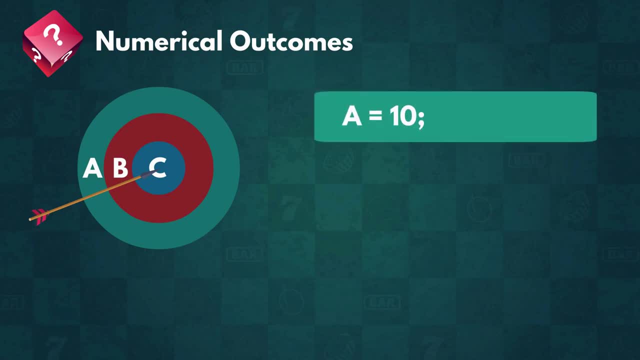 The outermost one is worth ten points, the second one is worth twenty points and the bull's-eye is worth one hundred. You have practiced this method enough to always be able to hit the target, but not so much that you hit the center every time. 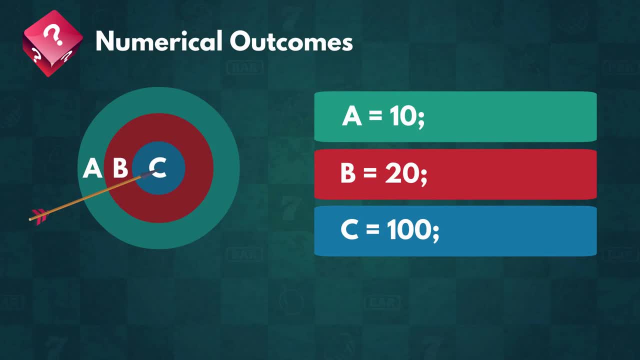 The probability of hitting each layer is as follows: 0.5 for the outmost, 0.4 for the second and 0.1 for the center. The expected value for this example would be 0.5 times ten. 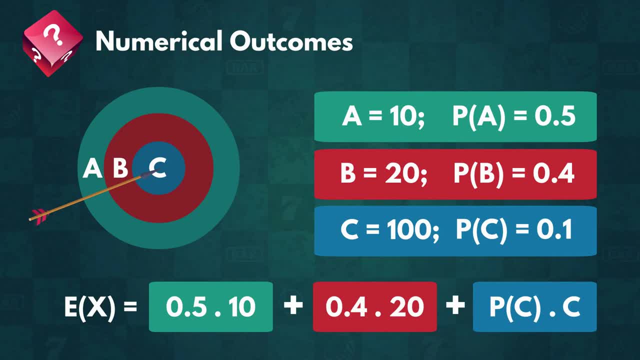 plus 0.4 times twenty plus 0.1 times one hundred, This is equal to five plus eight plus ten or twenty-three. Wait, We can never get twenty-three points with a single shot, So why is it important to know? 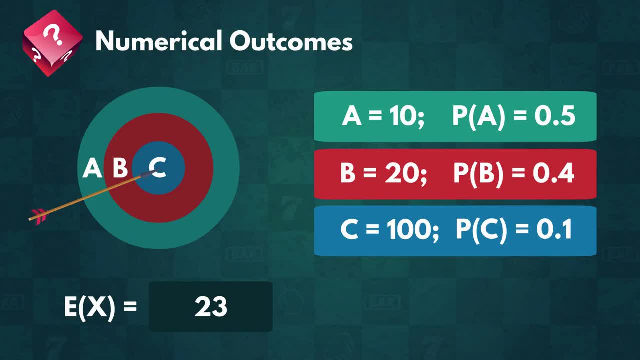 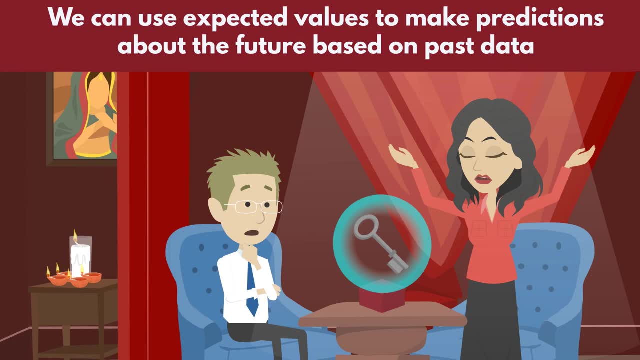 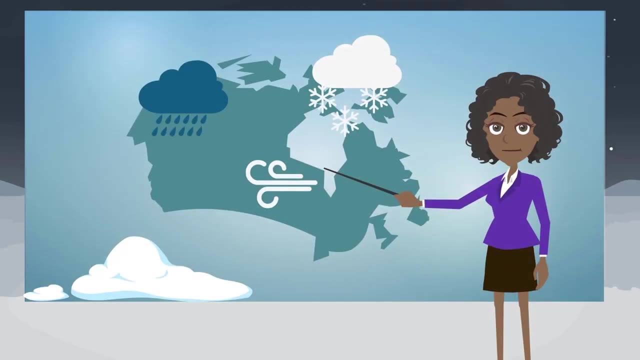 what the expected value of an event is. We can use expected values to make predictions about the future based on past data. We frequently make predictions using intervals instead of specific values due to the uncertainty the future brings. Meteorologists often use these when forecasting the weather. 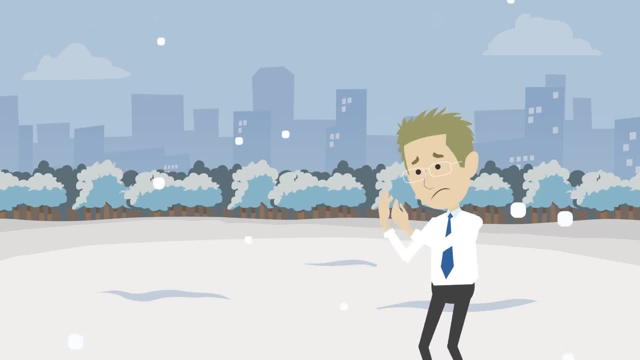 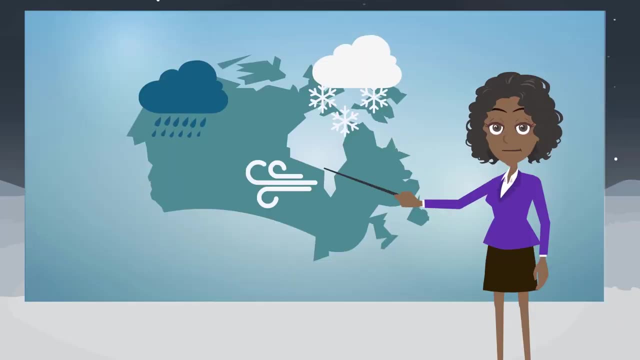 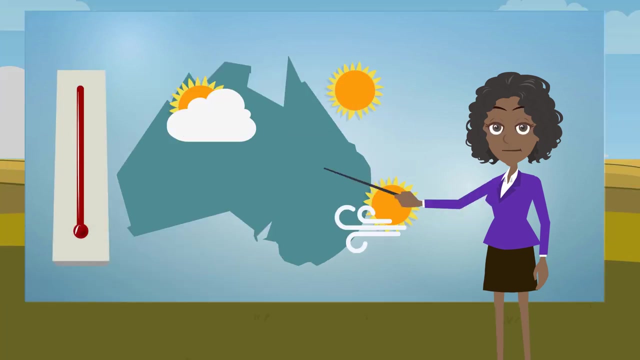 They do not know exactly how much snow, rain or wind there is going to be, so they provide us with likely intervals instead. That is why we often hear statements like expect between three and five feet of snow tomorrow morning or temperatures rising up to ninety degrees on Wednesday. 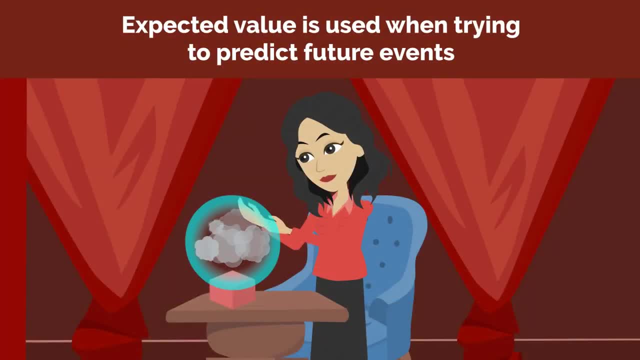 So far we have learned that the expected value is used when trying to predict future events. Sometimes the result of the expected value is confusing or doesn't tell us much. For instance, let us discuss a very famous example: throwing two standard six-sided dice. 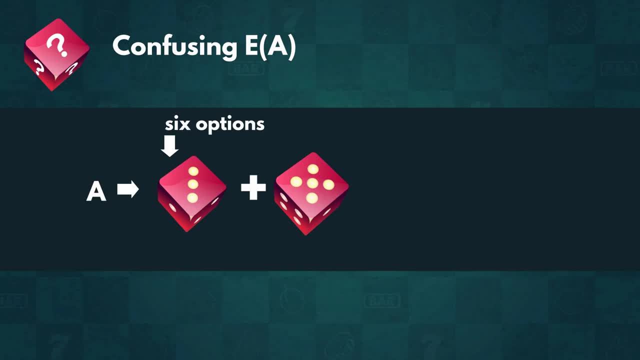 and adding up the numbers on top, We have six options for what the result of the first one could be. Regardless of the number we roll, we still have six different possibilities for what we can roll on the second die. That gives us a total of six times six. 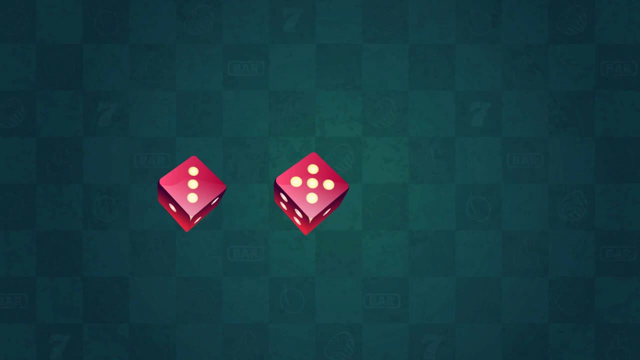 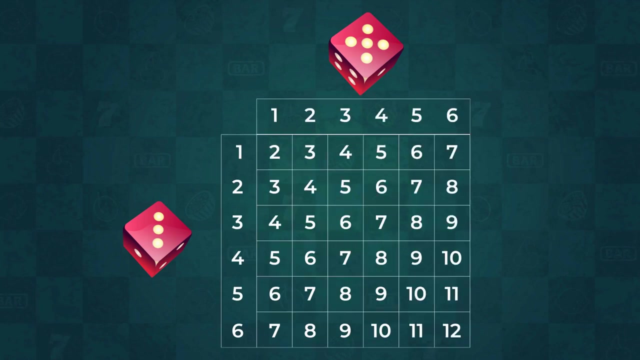 equals thirty-six different outcomes for the two rolls. For clarity, we can write out the results in a six by six table where we write the sum of the two dice. You can clearly see that we have repeating entries along the secondary diagonal and all diagonals parallel to it. 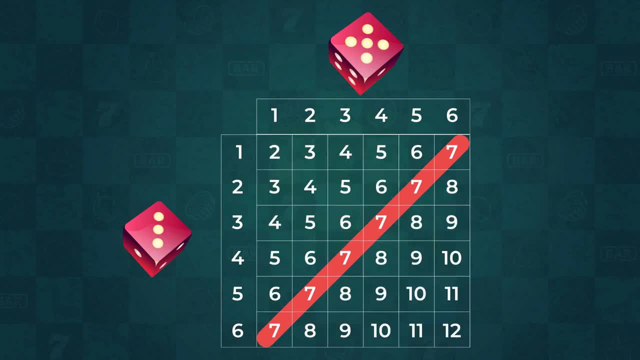 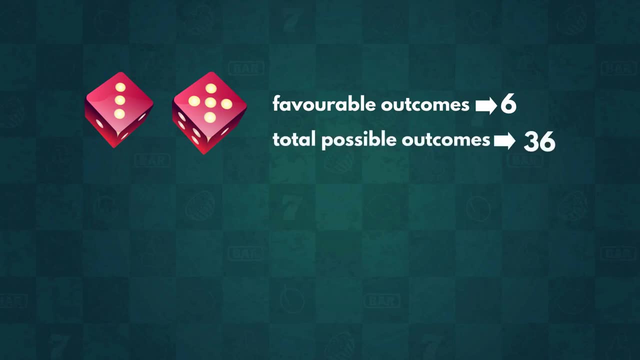 Notice how seven occurs six times in the table. This means we have six favorable outcomes. As we already mentioned, there are thirty-six possible outcomes, so the chance of getting a seven equals six over thirty-six or just one six. Let's also compute the expected value for this event. 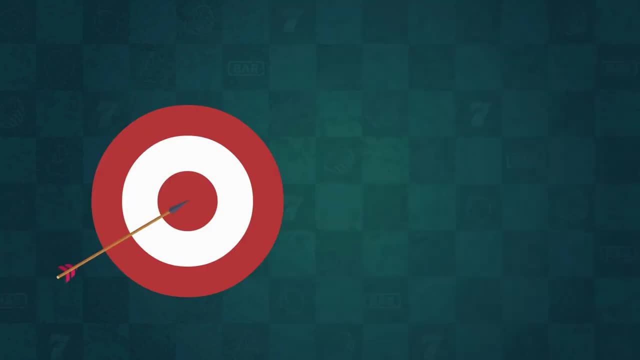 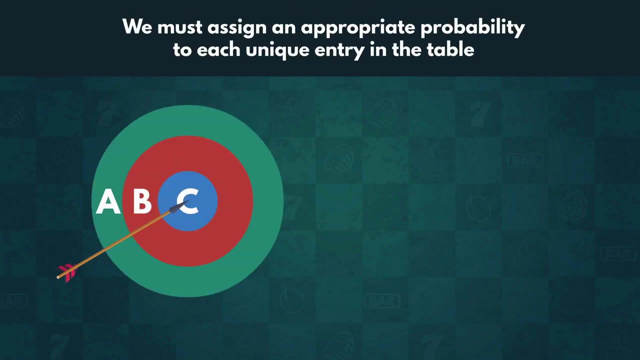 Since we are dealing with numerical data, we should apply the same formula we used for the archery problem. To do so, we must assign an appropriate probability to each unique entry in the table, Just like with the sum being seven. we do that based on the number of times. 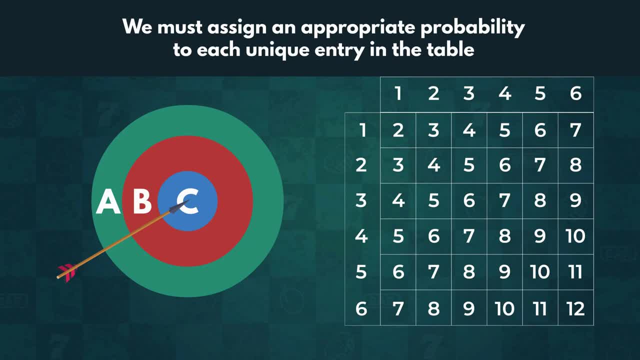 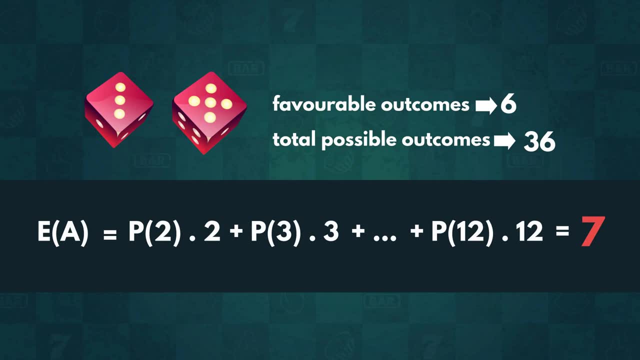 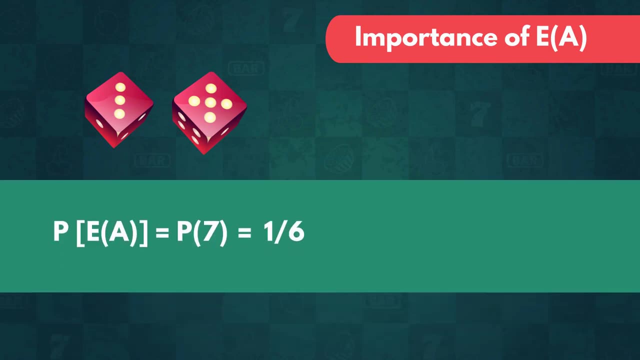 the number features in the table. If we do so, we are going to get the expected value, which ends up being seven. But how important is this value if the probability associated with it is only one sixth? The sum being equal to seven might be the most probable answer. 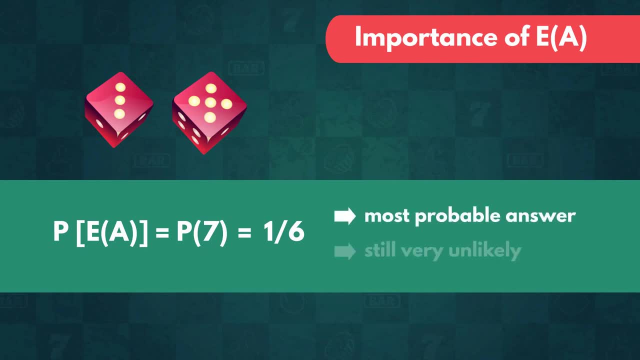 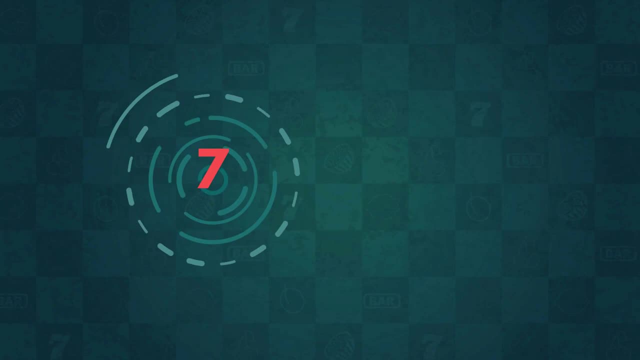 but it is still very unlikely to occur. Thus, we cannot reasonably bet on getting a sum of exactly seven. Moreover, even though we are suggesting seven is the most probable sum, how can you be sure? What we can do is to create a probability frequency distribution. 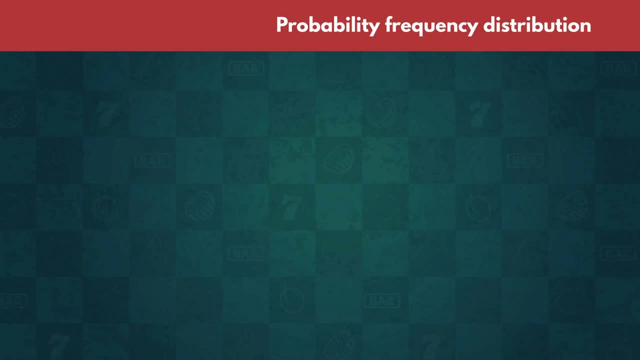 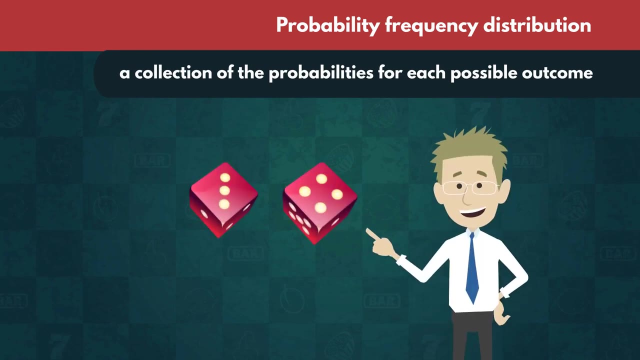 Simply put, a probability frequency distribution is a collection of the probabilities for each possible outcome. That's how I know that seven was the most probable sum of two dice. Usually it is expressed with a graph or a table To understand what a probability frequency distribution. 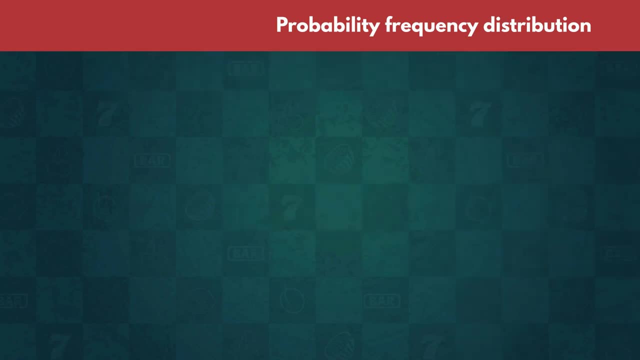 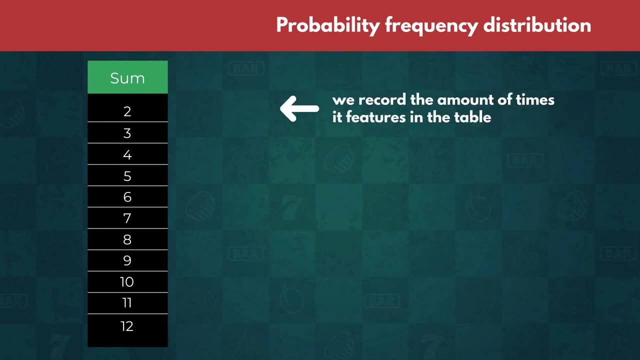 looks like we are going to construct one right now, Using the sample space table we already constructed. for each unique sum, we record the amount of times it features in the table. This value is known as the frequency of the outcome, For example. 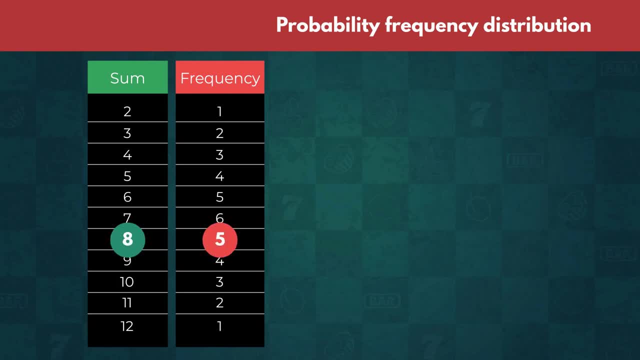 getting a sum of eight in five different cases means that eight has a frequency of five. OK, If we write out all the outcomes in ascending order and the frequency of each one, we construct a frequency distribution table. By examining this table, we can easily see: 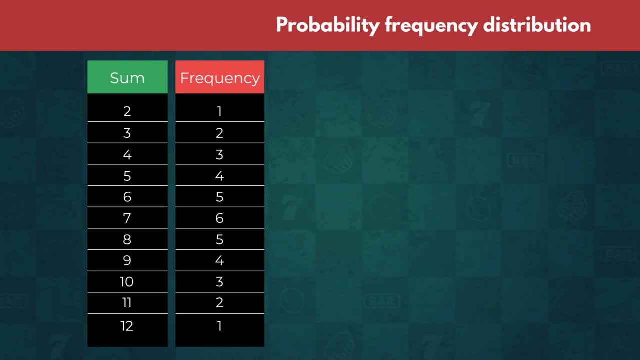 how the frequency changes with the results. Good job. At this point, we've done most of the work. The final step in getting the probability frequency distribution might be the most intuitive one. We need to transform the frequency of each outcome into a probability. 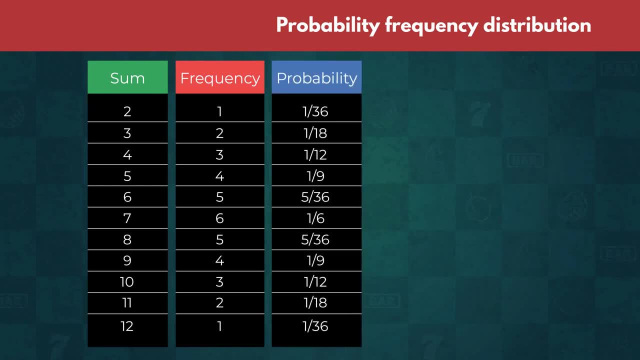 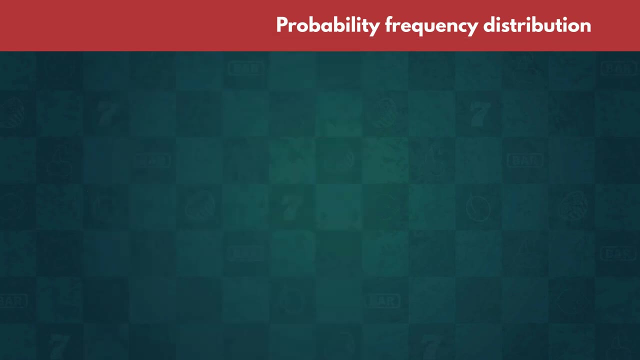 Knowing the size of the sample space, we can determine the true probabilities for each outcome. We simply divide the frequency for each possible outcome by the size of the sample space. A collection of all the probabilities for the various outcomes is called a probability frequency distribution. 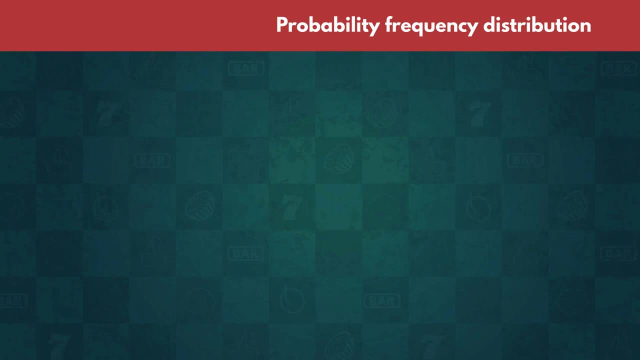 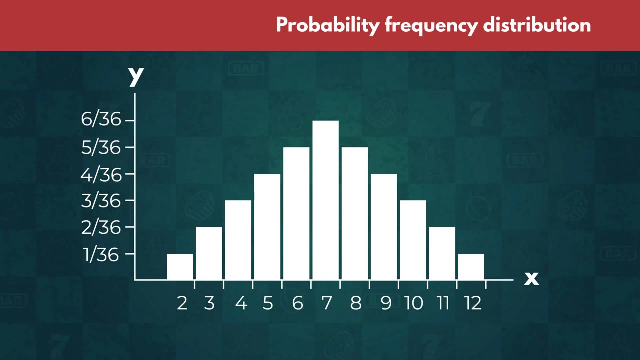 As mentioned earlier, we can express this probability frequency distribution through a table or a graph. All right On the graph we see the probability frequency distribution. The x-axis depicts the different possible numbers of spades we can get and the y-axis represents the probability. 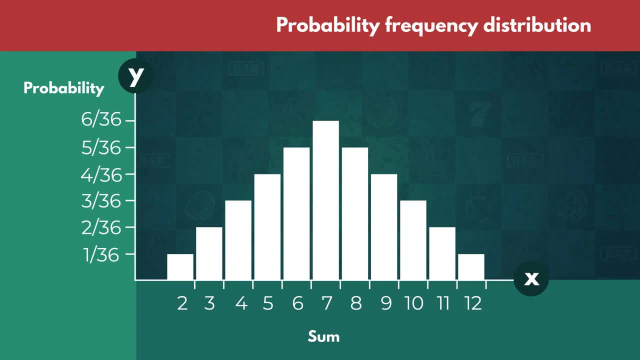 of getting each outcome. When making predictions, we generally want our interval to have the highest probability. We can see that the individual outcomes with the highest probability are the ones with the highest bars in the graph. Usually, the highest bars will form around the expected value. 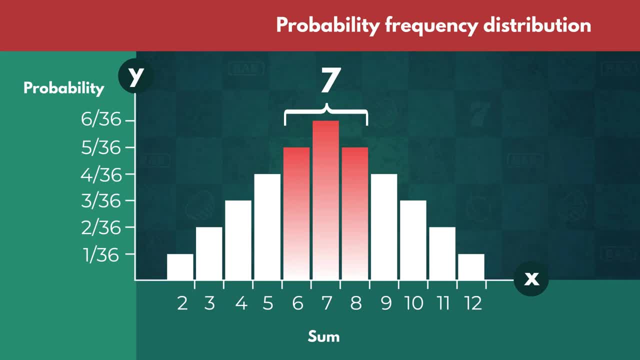 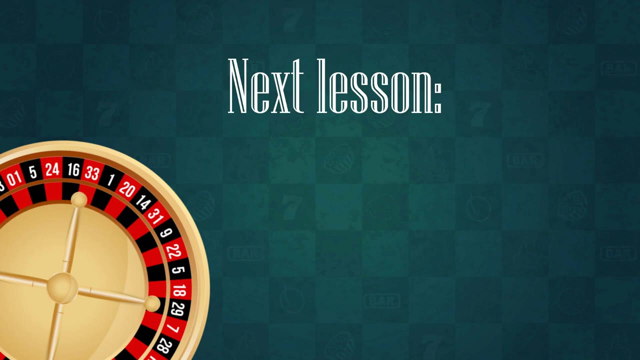 Thus the values around it would also be the values with the highest probability. This suggests that if we want the interval with the highest probability, we should construct it around the expected value. Before we move on to the next section, we need to talk about the opposite of an event. 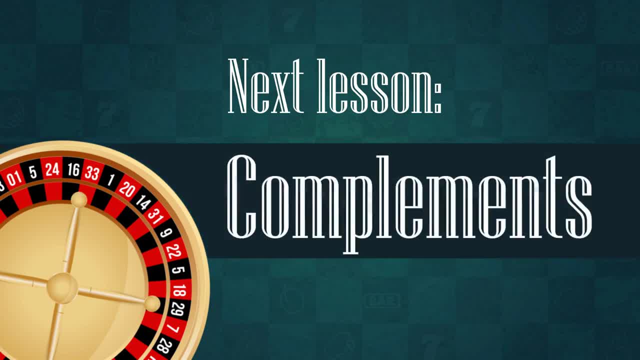 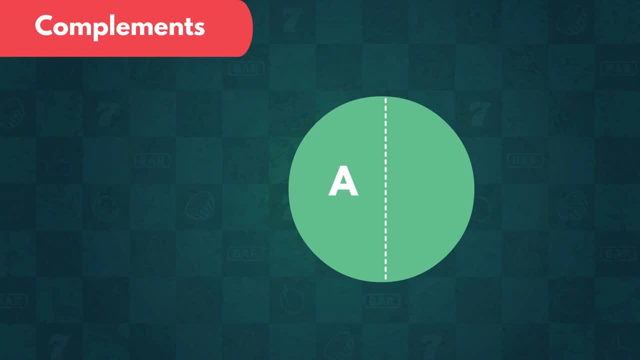 The term we use in probability theory is the complement, and we are going to explain why it is so important in the next lecture. Let's talk about some of the characteristics of probabilities and events. For starters, let's define what a complement is. 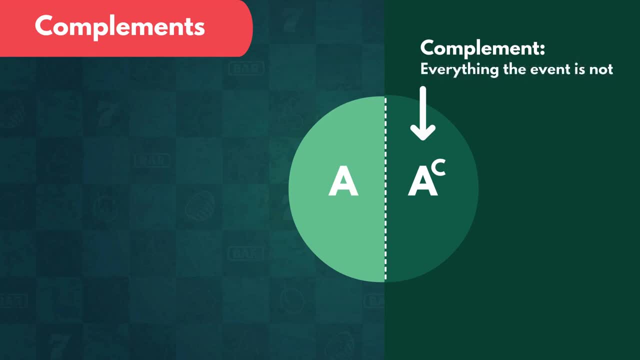 Simply put, a complement of an event is everything the event is not As the name suggests. the complement helps complete the rest of the sample space. To calculate the probability of the complement of an event, we need to set up a few things. 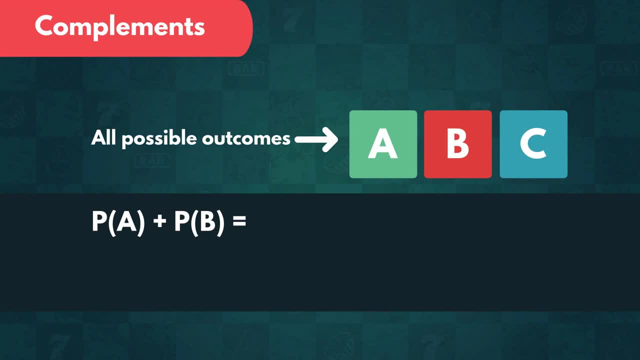 For starters, if we add the probabilities of different events, we get their sum of probabilities. Now, if we add up all the possible outcomes of an event, we should always get 1.. Remember that having a probability of 1 is the same as being 100% certain. 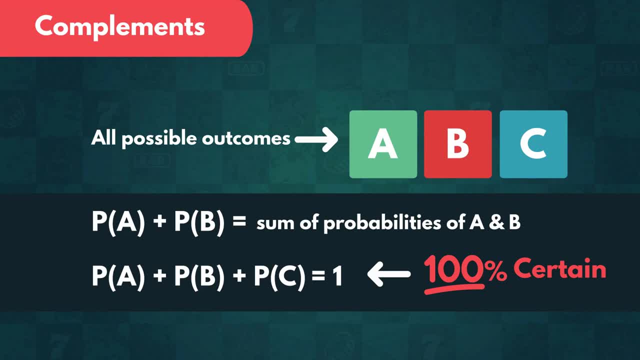 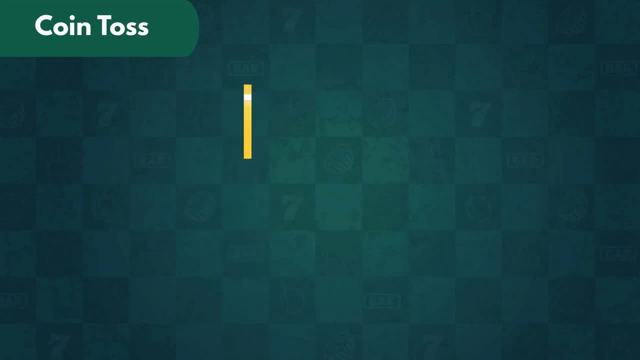 We are going to explain why this is true with several examples. Okay, imagine you are tossing a coin. When it falls, we are guaranteed to get either heads or tails. Therefore, if we account for the sum of all the probabilities of getting heads or tails, 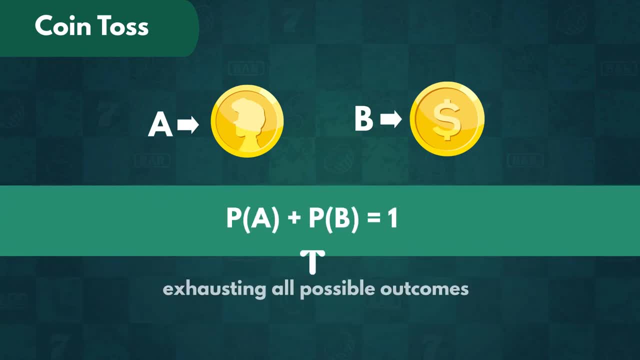 we have completely exhausted all possible outcomes. We have accounted for the entire sample space, so we are 100% certain to get one of the two. Since we are certain one of these will occur, the sum of their probabilities should be 1.. 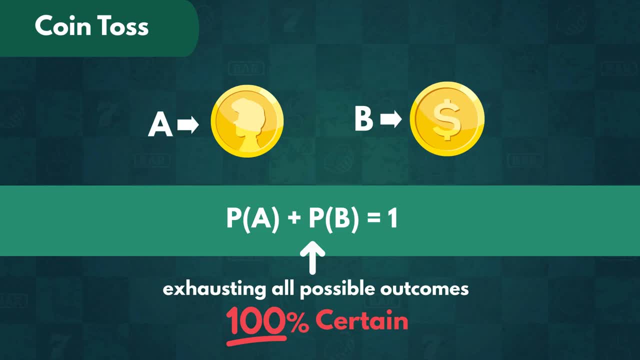 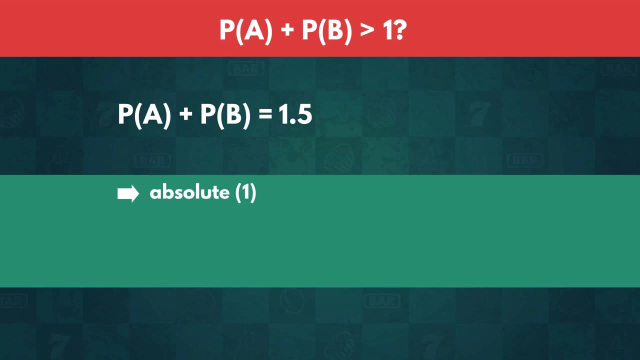 So what would it mean if we have a sum of probabilities greater than 1?? Recall that probability of 1 expresses absolute certainty By definition. we cannot be any surer than being absolutely sure, so a probability of 1.5 does not make intuitive sense. 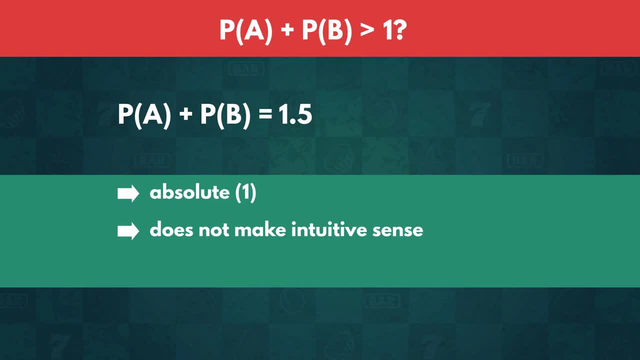 Instances where we can get such a sum of probabilities is when some of the assumed outcomes can occur simultaneously. This means we are double counting some of the actual possible outcomes. Now, another peculiar case is if we end up with a sum of probabilities less than 1.. 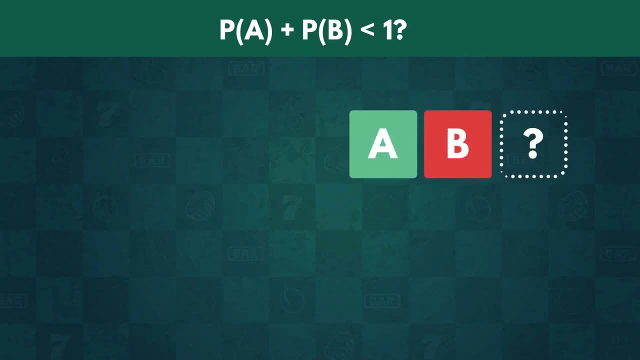 Then we have surely not accounted for one or several possible outcomes. Probability expresses the likelihood of an event occurring, so any probability less than 1 is not guaranteed to occur. Therefore, there must be some part of the sample space we have not yet accounted for. 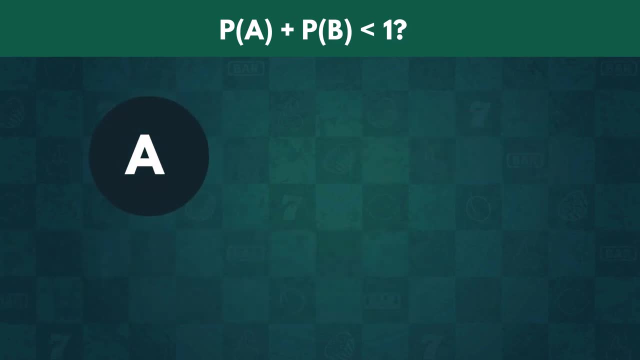 Great. Before we move on, we want to tell you that all events have complements and we denote them by adding an apostrophe. For example, the complement of the event A is denoted as A apostrophe. It is also worth noting. 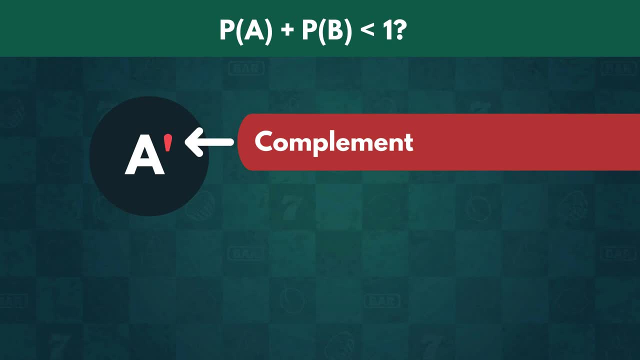 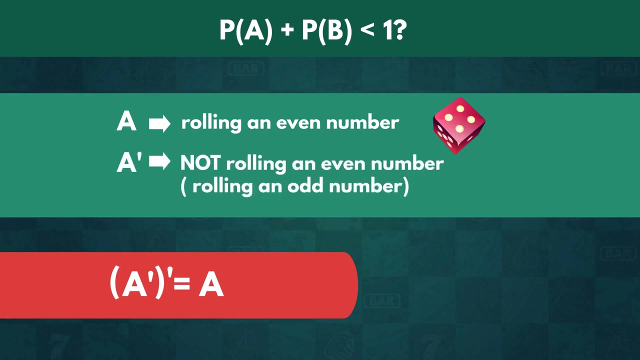 that the complement of a complement is the event itself. so A apostrophe, apostrophe would equal A. Now imagine if you were rolling a standard six-sided die and want to roll an even number. The opposite of that would be not rolling an even number. 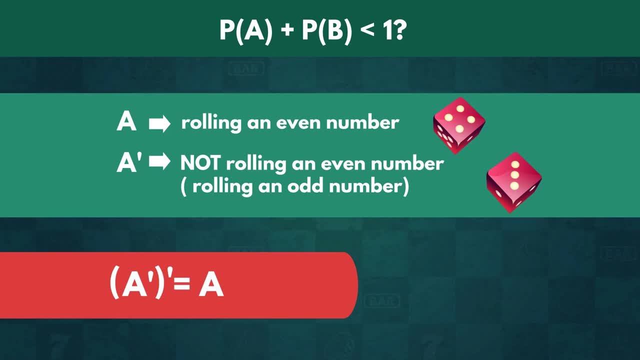 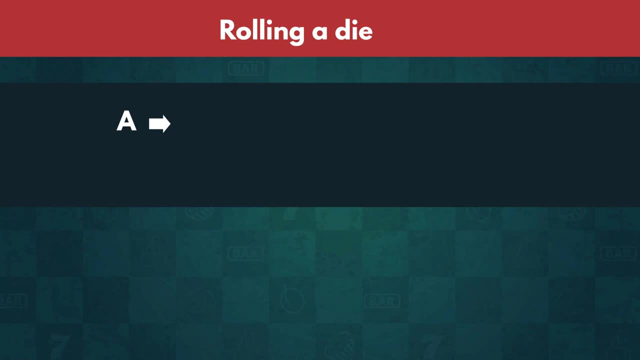 which is the same as wanting to roll an odd number. Complements are often used when the event we want to occur is satisfied by many outcomes. For example, you want to know the probability of rolling a 1,, 2,, 4,. 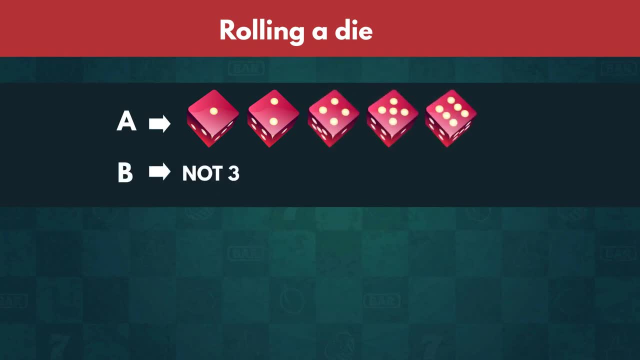 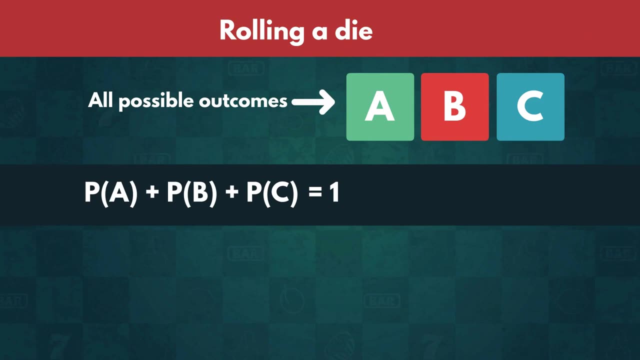 5, or 6. That is the same as the probability of rolling a 3.. This concept is extremely useful. We already said that the sum of the probabilities of all possible outcomes equals 1.. So you can probably guess how we calculate. 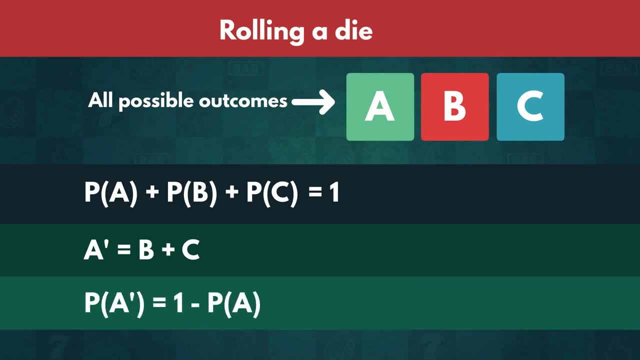 complements The probability of the inverse equals 1 minus the probability of the event itself. To make sure you understand the notion well, we will look at the example we mentioned earlier: The sum of probabilities of getting 1,, 2,, 4,.